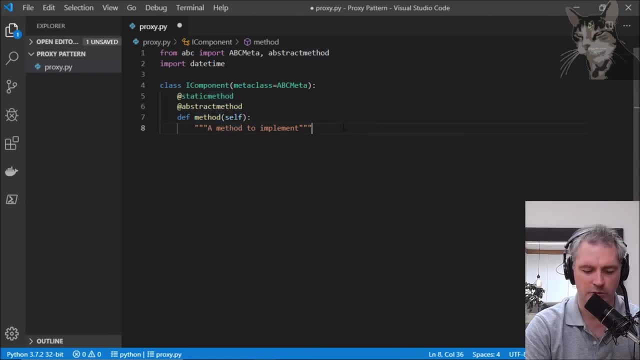 abstract with a method that should be implemented. Here's a component that implements the iComponent interface. There's the method and it just prints: the method has been called. So we can test that quickly by creating a little client component equals component componentmethod. Let's run that. 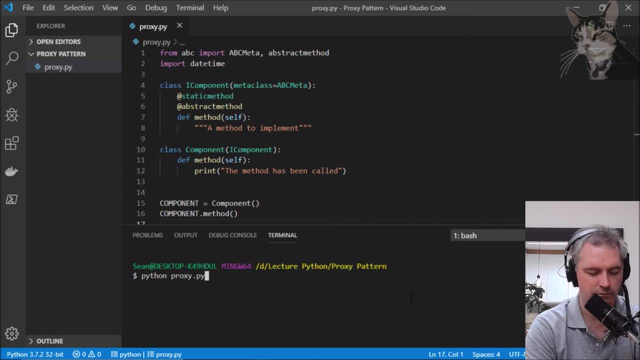 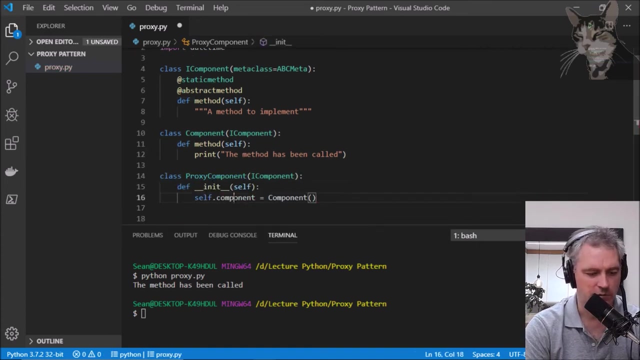 pythonproxypy. the method has been called. Let's create a proxy class. proxy component implements the i component interface. We'll need an init where it creates its own internal component and we'll need to implement the method method. and here I can just call directly: self component dot method. 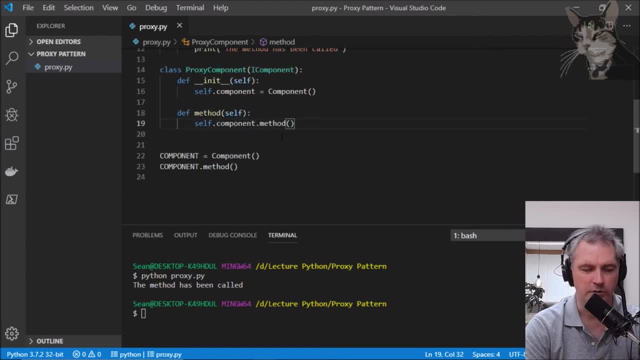 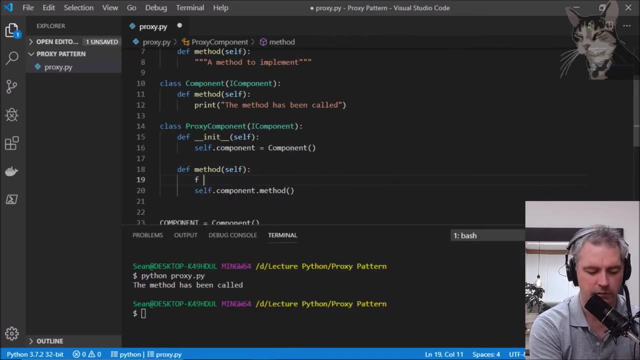 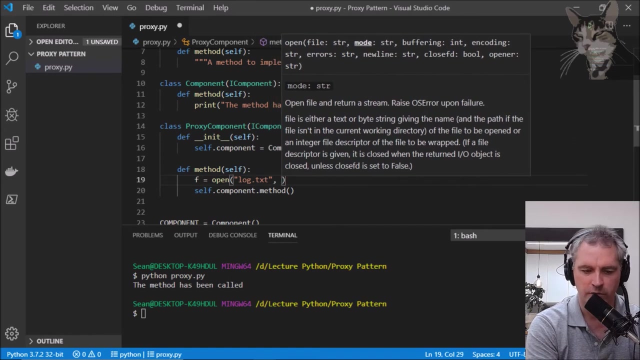 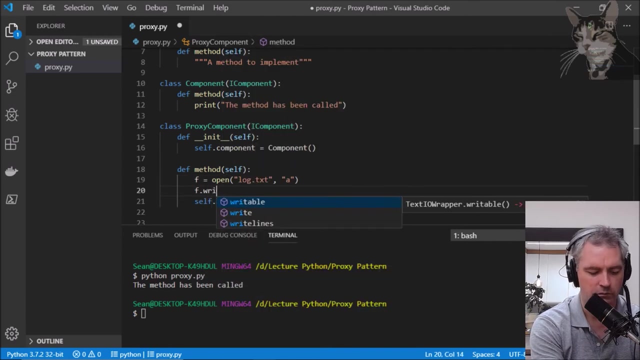 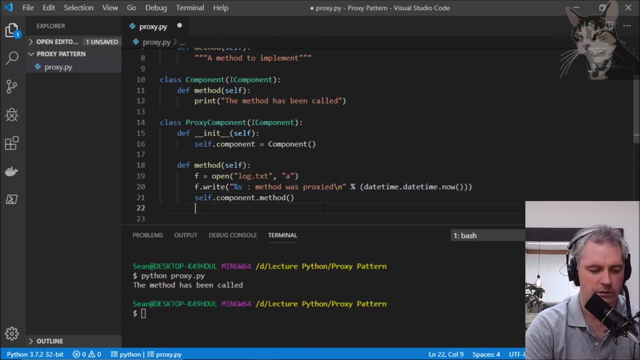 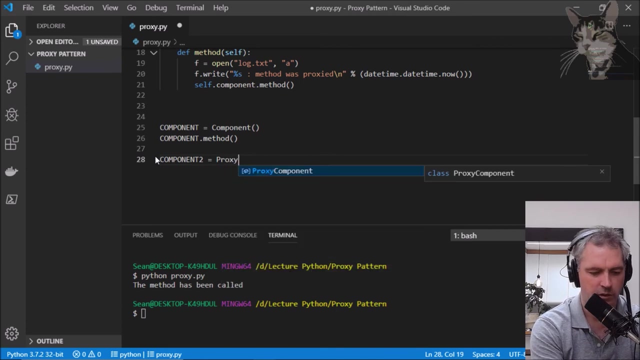 And that is proxied, but it's not really doing anything. I wanted to just want to extend it, so I'm also going to log it. So f equals open log dot text for appending f dot. write method was proxied and the date now Okay, so let's try that out. so let's make that another component. two equals a proxy component. 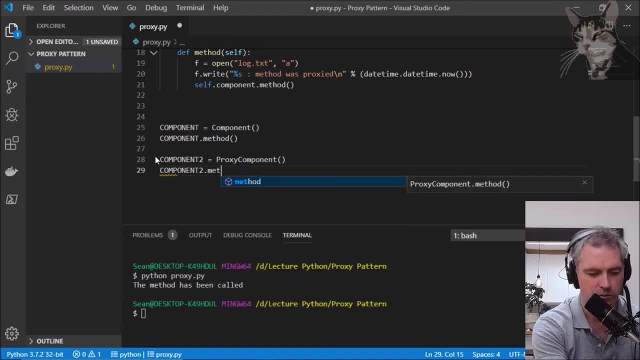 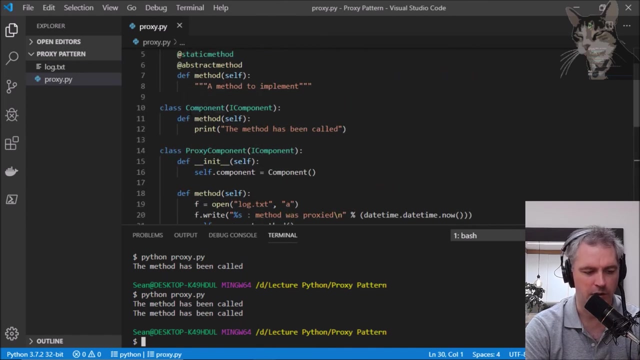 component two: dot method. Let's see what happens when we run that python proxypy. So the same component, the underlying same underlying component, was called both times, except in the second time this extra logging functionality was executed. So we can see it was written to log dot text. there's log dot text was proxied. 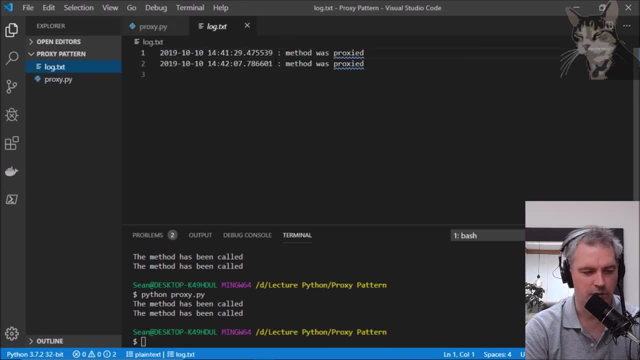 Let's try that again. there we go, log dot text and try it again, and each time the proxy method is called we get a new log. that's the proxy pattern implemented as a logger.